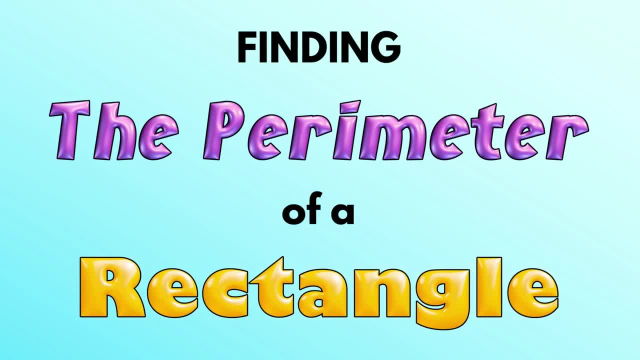 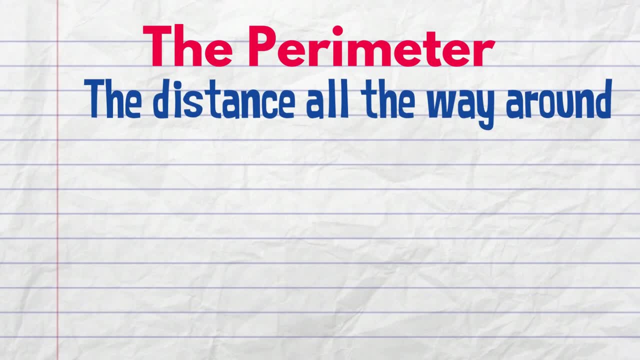 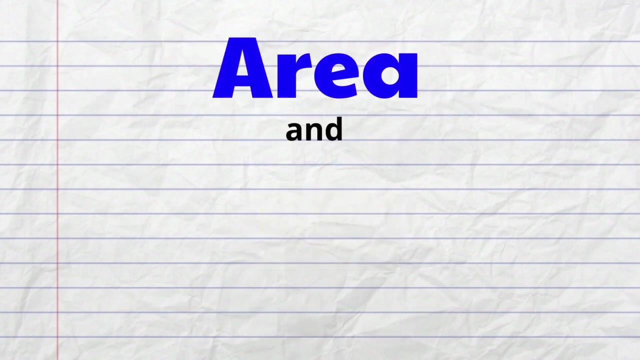 Finding the perimeter of a rectangle: 3 strategies you can use. The perimeter is the distance all the way around the outside of something. The lines that make up this rectangle are the perimeter. The space inside is the area. Area and perimeter are a big deal in mathematics. 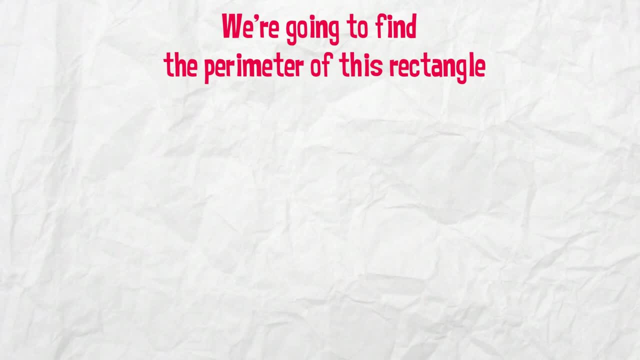 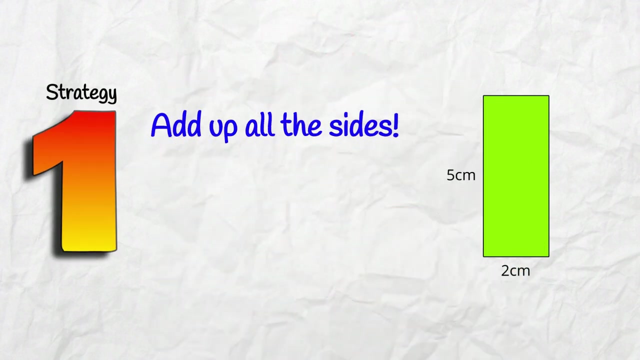 We're going to find the perimeter of this rectangle. We have 2 pieces of information: The length and the width, And that's all we need. These 2 sides are equal, So that's 5 plus 5. And these 2 sides are equal. 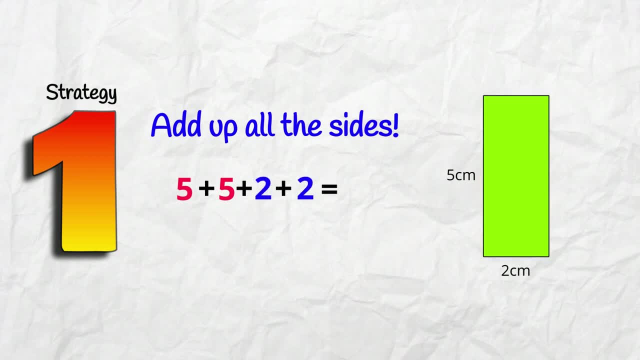 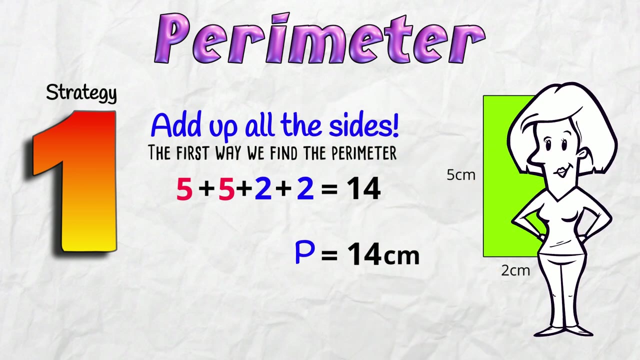 2 plus 2. All together that makes 14.. So the perimeter, or just P, is 14cm. Adding up all 4 sides is the first way we find the perimeter. Let's keep going and take a look at strategy number 2.. 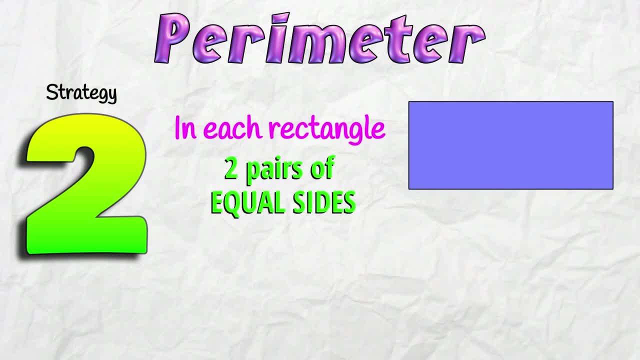 In each rectangle we have 2 pairs of equal sides, 2 lengths the same and 2 widths the same, So we can use doubling as a strategy. The length is 7cm, Double 7 is 14.. The width is 3cm. 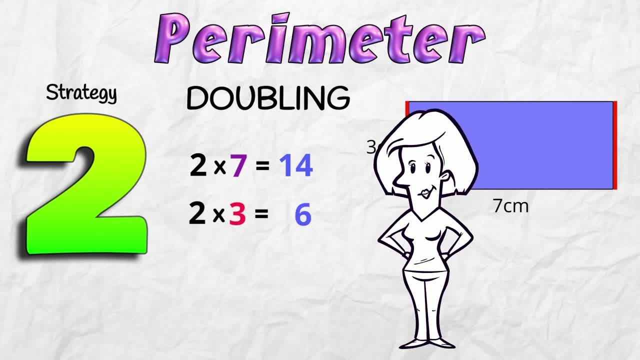 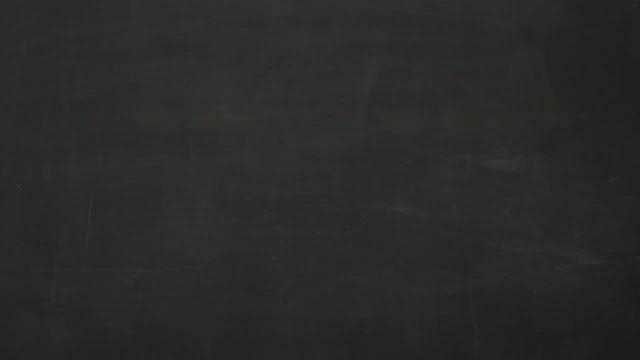 Double 3 is 6.. Next add up these doubled values to get the perimeter: 14 plus 6 is 20.. The perimeter is 20cm. There's a math formula to show what we just did. A formula is just a written description that shows what to do. 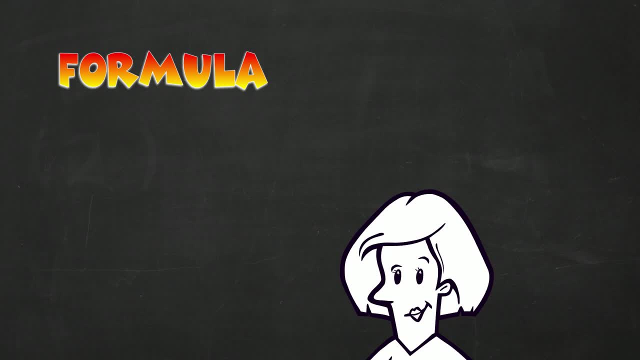 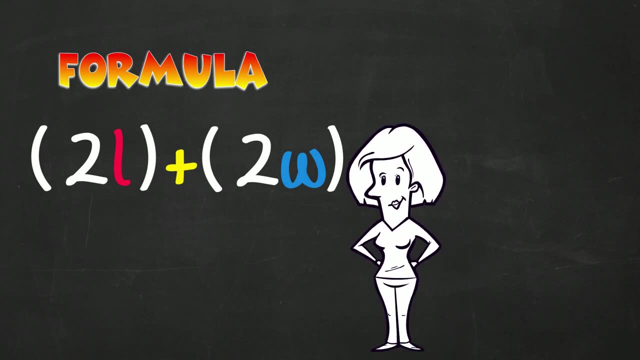 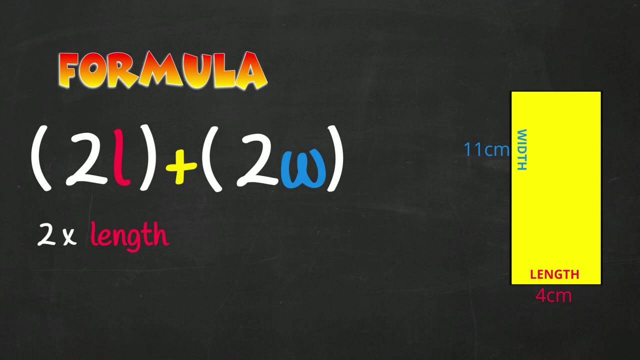 The formula for this strategy is 2L plus 2W. We make sense out of it by rewriting the formula using the measurements from the diagram. 2L means 2 times the length, So 2 times 4.. 2W is 2 times the width. 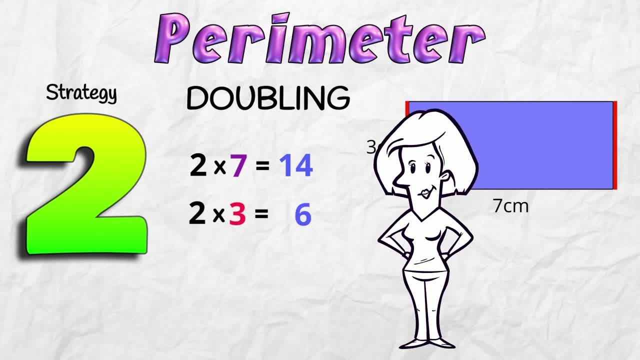 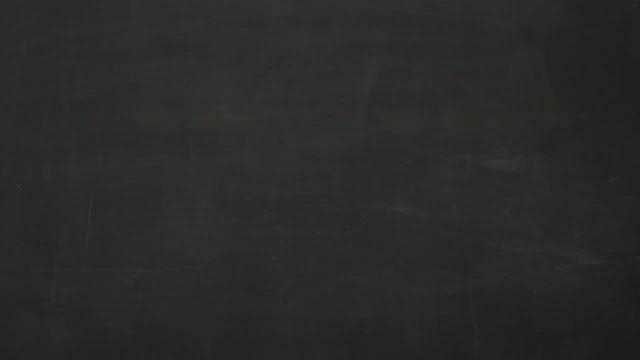 Double 3 is 6.. Next add up these doubled values to get the perimeter: 14 plus 6 is 20.. The perimeter is 20cm. There's a math formula to show what we just did. A formula is just a written description that shows what to do. 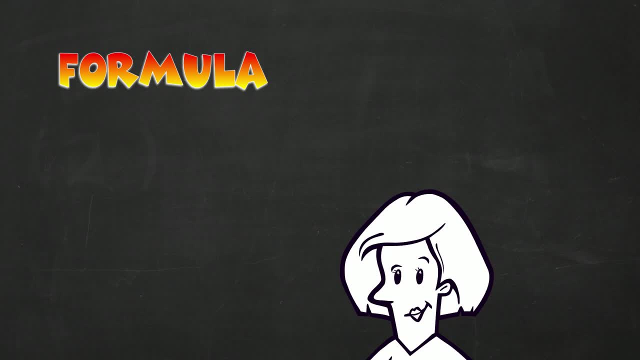 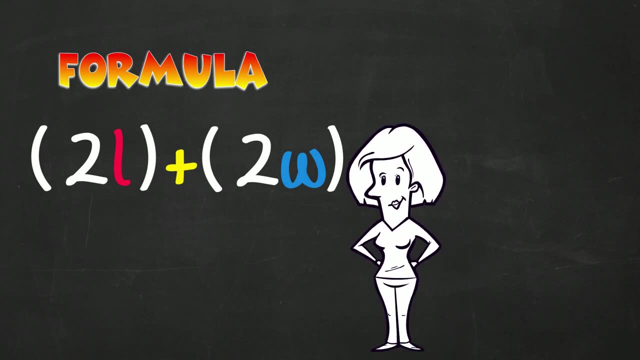 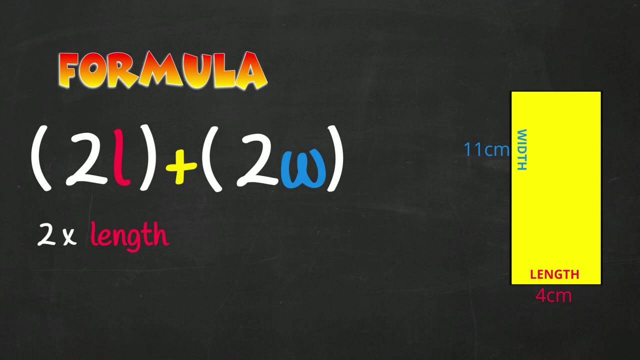 The formula for this strategy is 2L plus 2W. We make sense out of it by rewriting the formula using the measurements from the diagram. 2L means 2 times the length, So 2 times 4.. 2W is 2 times the width. 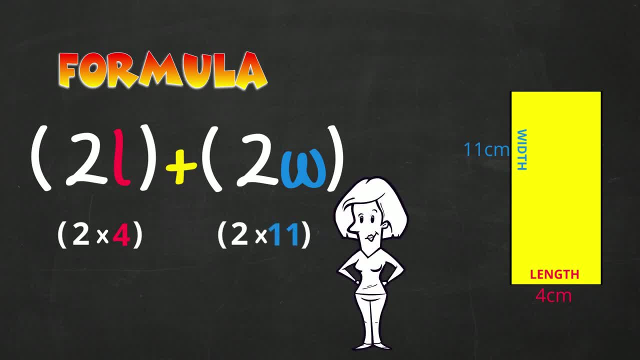 And that's 2 times 11.. And these parts are in brackets because of course we do those first and then we do the adding at the end. 2 times 4 is 8.. Plus 2 times 11 is 22.. 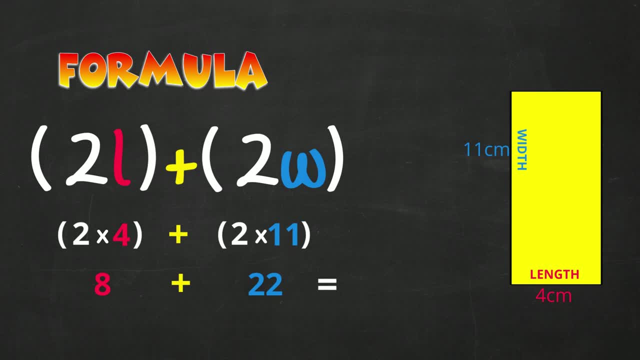 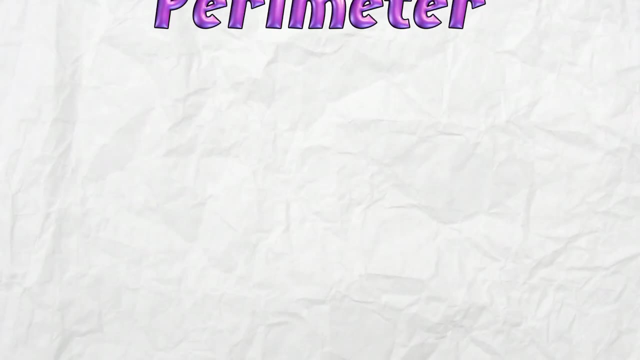 Then just add those figures together: 22 plus 8 is 30. The perimeter is 30cm. This formula clearly tells us what to do. You can do this Now. let's take a look at strategy number 3!. You can think of a rectangle as being made up. 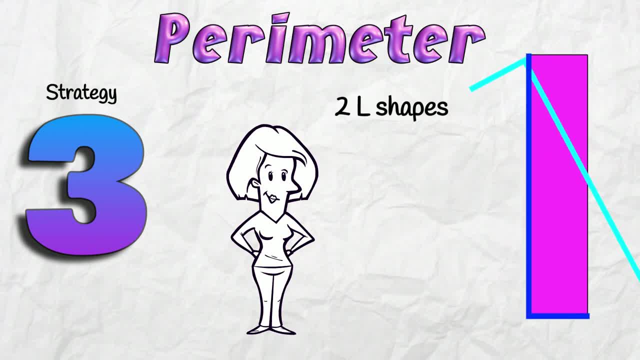 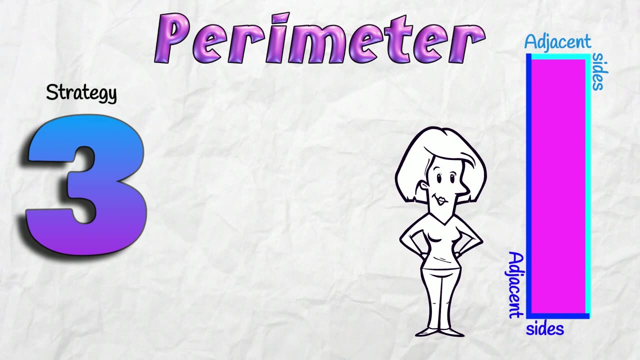 of 2 L shapes. These are called adjacent sides. Adjacent just means next to or adjoining. These sides are next to each other. They join at a corner. In strategy number 3, we start by adding 2 adjacent sides. So 2 plus 9 is 11.. 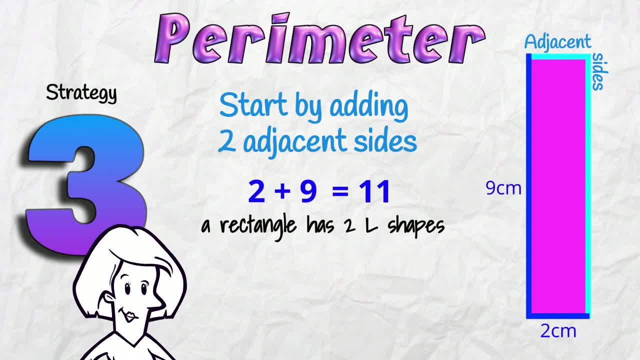 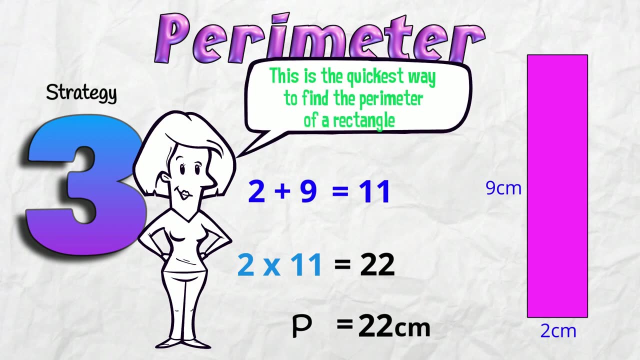 A rectangle has 2 L shapes, So we multiply by 2.. 2 times 11 is 22.. The perimeter is 22cm. This is the quickest way to find the perimeter of a rectangle: Just add 2 adjacent sides and double it. 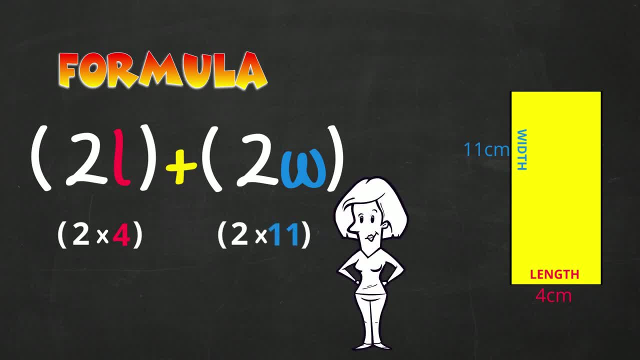 And that's 2 times 11.. And these parts are in brackets because of course we do those first and then we do the adding at the end. 2 times 4 is 8.. Plus 2 times 11 is 22.. 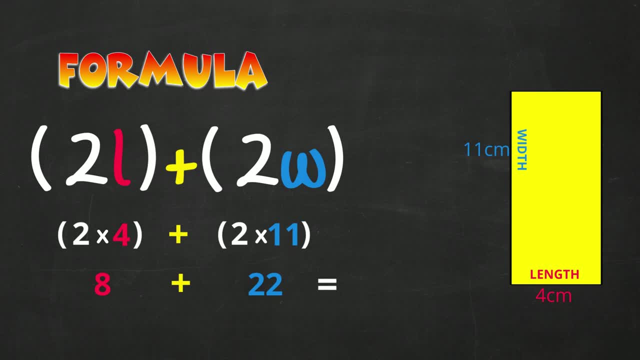 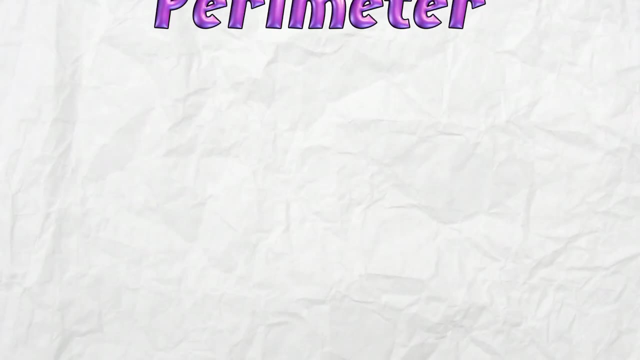 Then just add those figures together: 22 plus 8 is 30. The perimeter is 30cm. This formula clearly tells us what to do. You can do this Now. let's take a look at strategy number 3!. You can think of a rectangle as being made up. 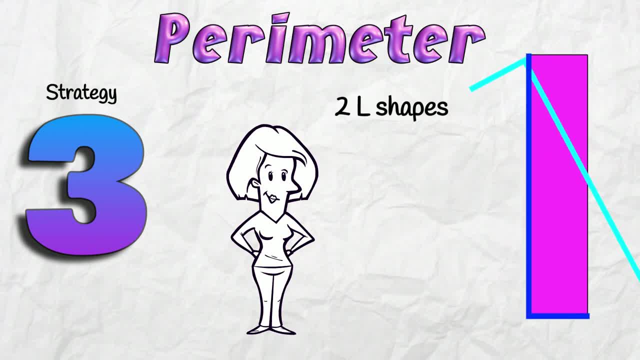 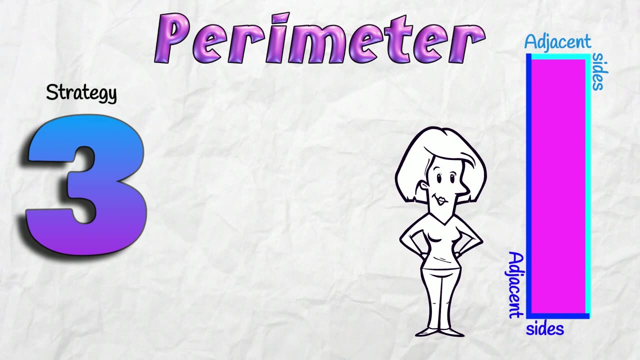 of 2 L shapes. These are called adjacent sides. Adjacent just means next to or adjoining. These sides are next to each other. They join at a corner. In strategy number 3, we start by adding 2 adjacent sides. So 2 plus 9 is 11.. 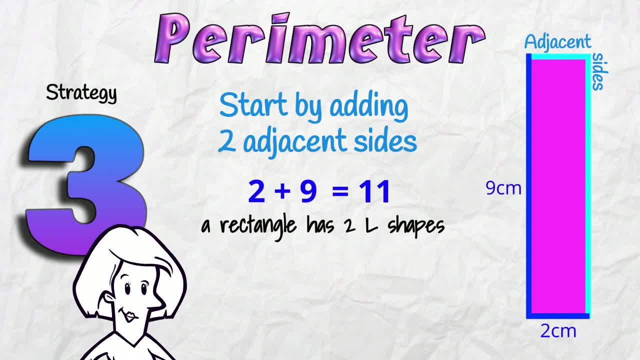 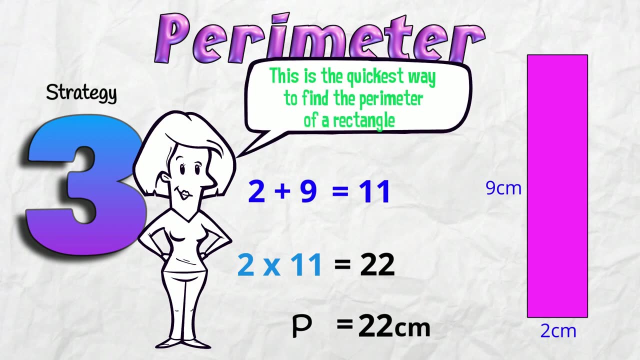 A rectangle has 2 L shapes, So we multiply by 2.. 2 times 11 is 22.. The perimeter is 22cm. This is the quickest way to find the perimeter of a rectangle: Just add 2 adjacent sides and double it. 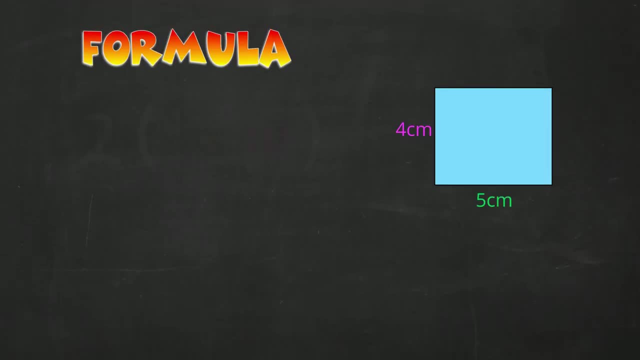 And there's a formula for this too: 2L plus W. The brackets are telling us to add the length and width first. The 2 outside the brackets tells us to multiply by 2.. And there's the perimeter. Don't forget to put the unit of measurement at the end. 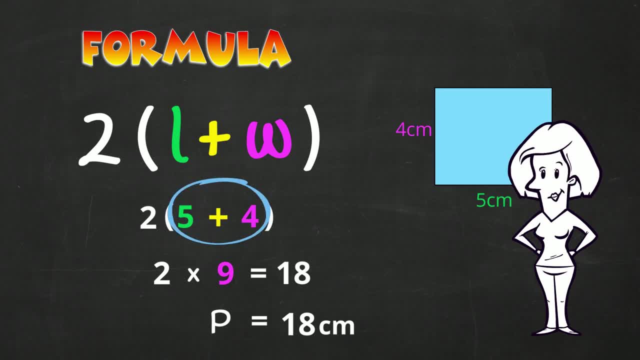 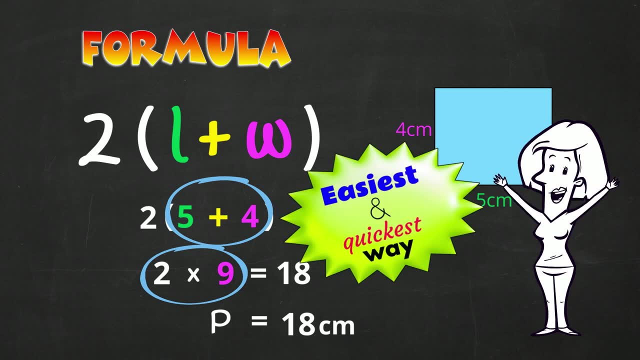 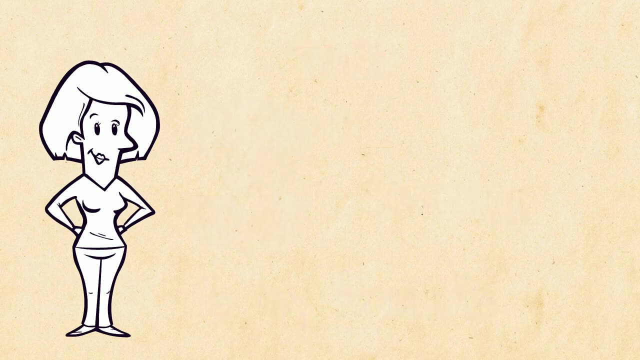 And, of course, this strategy only has 2 calculations to do. That makes this the easiest and quickest way to find the perimeter of a rectangle, And that's why this third strategy is my favourite. And now you've seen them all. You have 3 strategies you can use. 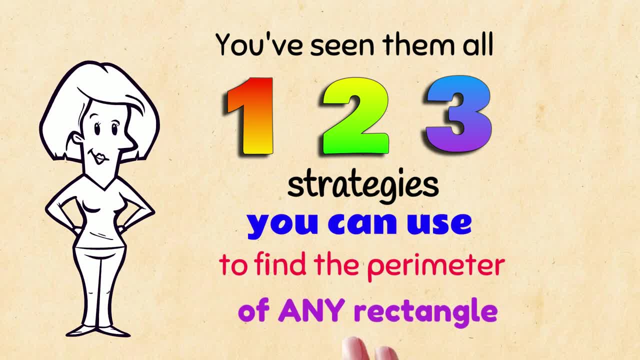 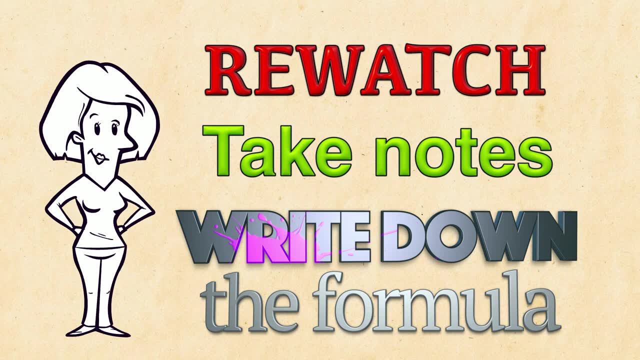 to find the perimeter of any rectangle. Rewatch and take notes, Write down the formula so you get used to using it. You are going to rock the perimeter of a rectangle.